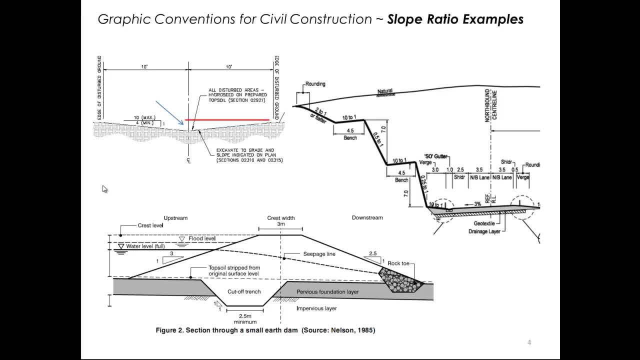 that topic further in another video, Beginning then at the upper left by my pointer here. this view is a simple swale, which a swale is just another name for a shallow drainage ditch. Note that in this case the slope ratio is given in both a minimum and maximum, and this is a little confusing, because the minimum is x and the minimum is a negative. So in this case the minimum is x-x, So the slope ratio is x-x and the minimum is x-x, So the minimum is x-x and the minimum is x-x. 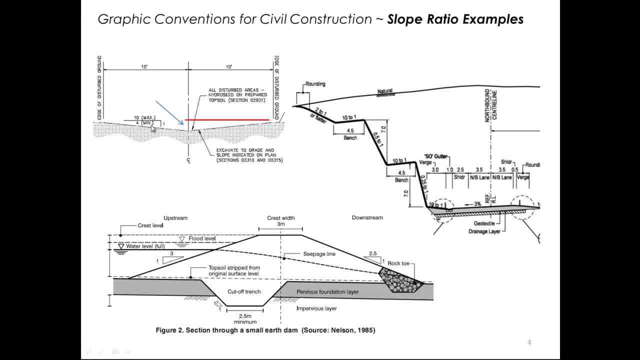 at a 4 to 1 is really the steepest allowable slope, and the maximum at 10 to 1 then would be the flattest allowable slope. Well, what would the maximum allowable depth be at the swale? Okay, this would represent a level line from the ground over to the center of the swale. so 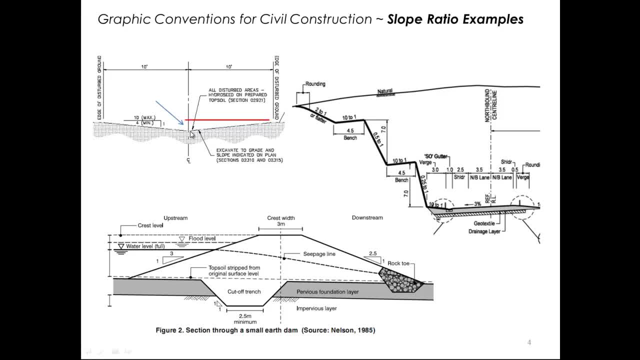 what would the maximum depth be at the center line of the swale, at the 4 to 1?? Well, it's 10 feet. so if we divide 10 by 4, that's 2.5, and 2.5 times 1 tells us that the distance from here to here. 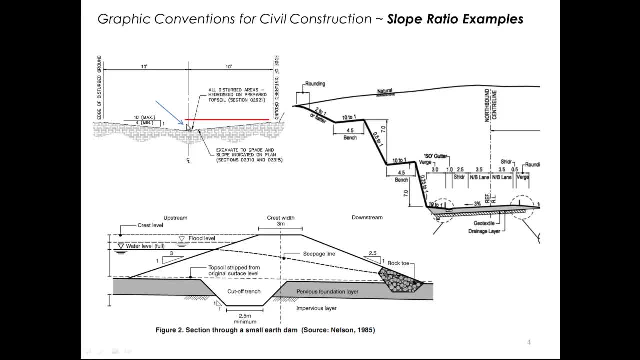 the depth at the swale at a 4 to 1 slope would be 2.5 feet, and if it were 10 to 1, obviously 10 feet, 1 foot. so this would be 1 foot deep here. Pretty neat, huh. Our second example to the right: 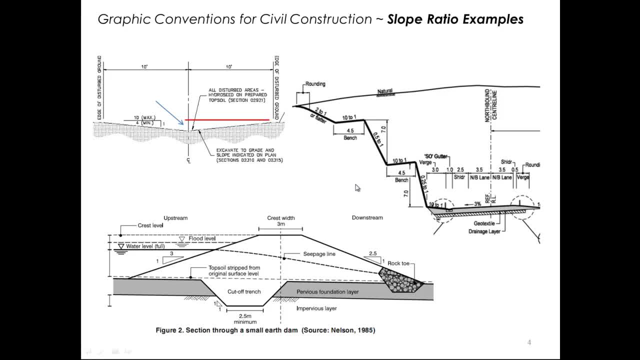 is another section view This time. this section is a row roadway excavation, most likely through a hill and probably with blasted rock, because we see these very steep slopes. We can see one line of the pavement shown down on the bottom here, one lane of the of the two-lane road. So let's start in the upper left corner where it says: 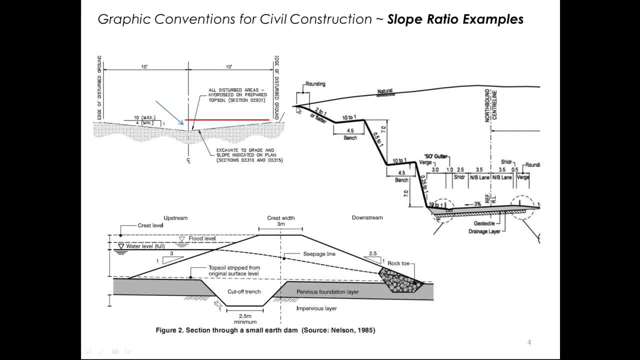 rounding As the excavation begins, there's a 2 to 1 slope or flatter. this would depend on the nature of the material, but definitely they're in soil here and then there's a little reverse slope of a 10 to 1 and the idea is that any soil that might erode would be caught on the backside of. 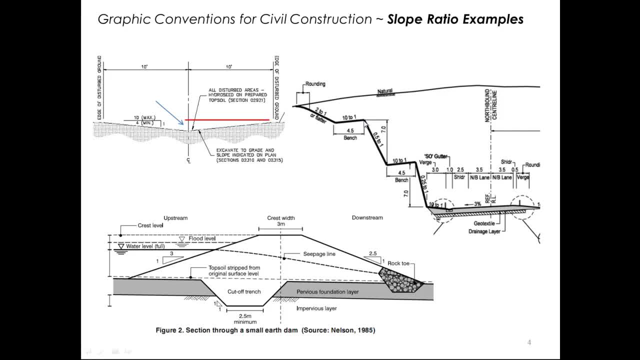 that slope and then, as the rock is encountered, the slope steepens to a. it says 0.5, that's a half to 1. okay, so for seven foot of depth, a half to one, then another ten to one bench, four and a half foot, and then a quarter to one on down to the bottom here, and then a ten to one. so this would: 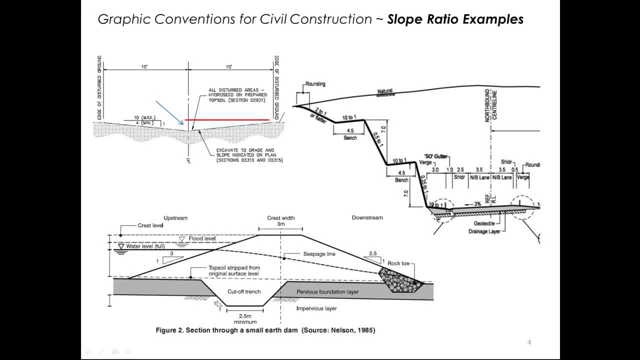 tell the contractor exactly how this cut through this hill and through this rock would be excavated. Our last example is a simple earth dam and again let me get a highlighter here and again we can see how this convention is used. The water side slope of the dam is a three to one, the 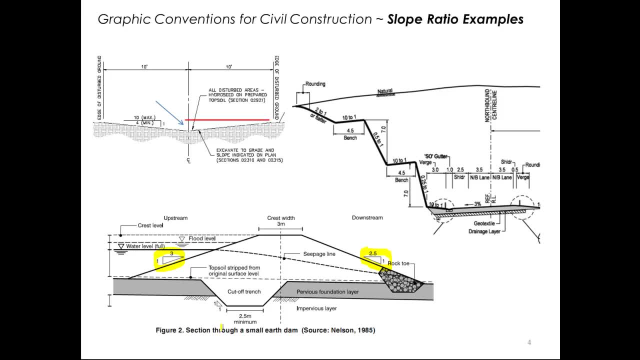 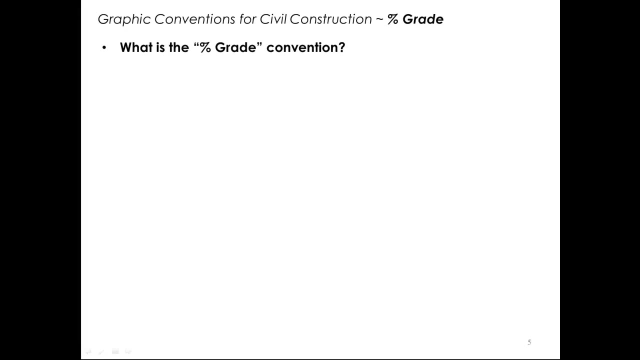 backside slope of the dam is a two and a half to one. in the trench that holds the and ties the dam into the rock underneath the dam is a one to one. Let's move on and take a look, then, at the percent grade convention. Remember, we said that this 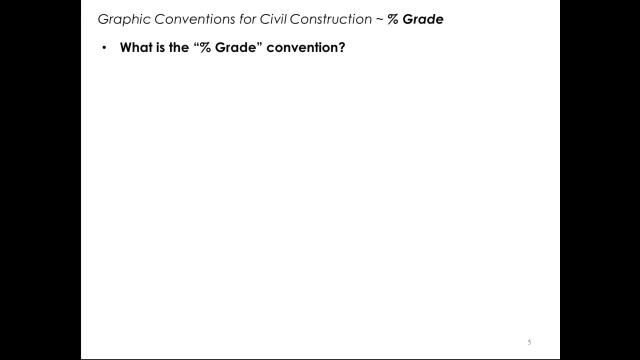 method was used to specify more gradual inclination and or for longer distances. Percent grade is defined simply as the vertical change in feet over a constant 100-foot horizontal distance, The vertical change in feet over a constant 100-foot horizontal distance. And here we see a graphic example that we have three foot vertical in 100 feet. remember the. 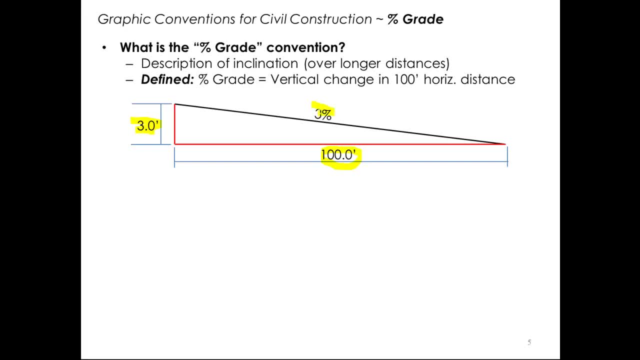 hundred is the constant, so three and a hundred tells us then that this is a three percent gradient. Sometimes we need to find what the actual percent gradient is. So let's look at another example, and in this case we've got a vertical rise of four point three feet. 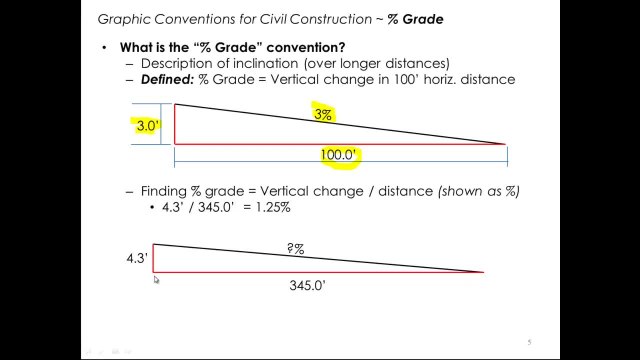 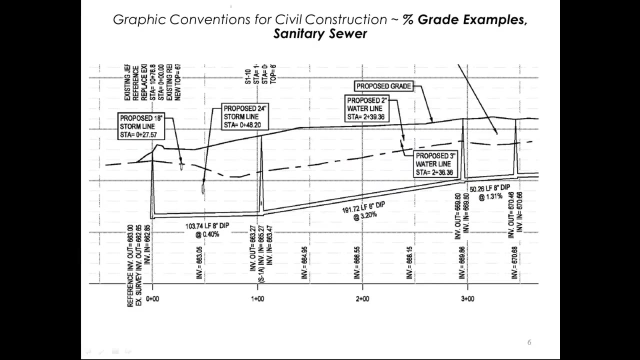 and we've got a horizontal run of three hundred and forty five feet. So we simply divide the rise by the run and we find in this case that our slope is one point two five percent. Let's look at an example then from a plan. 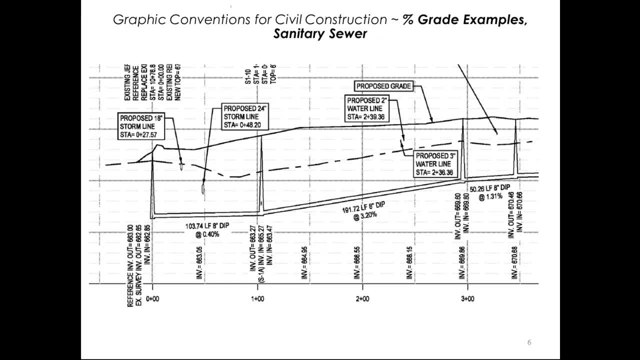 in this case we're looking at a sanitary sewer profile and note- let me get the highlighter- note, then, how the gradient for each run between these are manholes, how the gradient for each run varies and how it is specified in the profile view to two decimal places. let's find another. 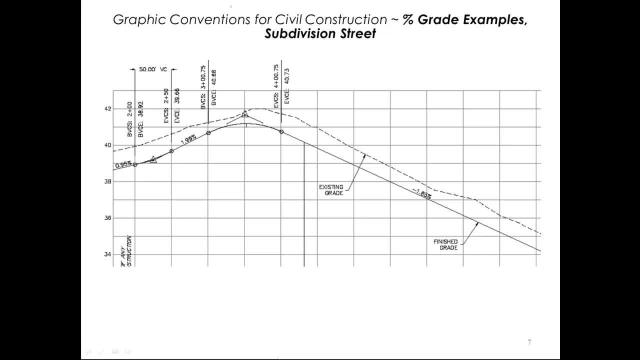 example, and in this case we're looking at a street profile. well, this looks about like a roller coaster if you just look at it the way it's drawn. what the situation is is that normally, in profile views, an exaggerated scale is used, and we talked about this in another video, so it's really 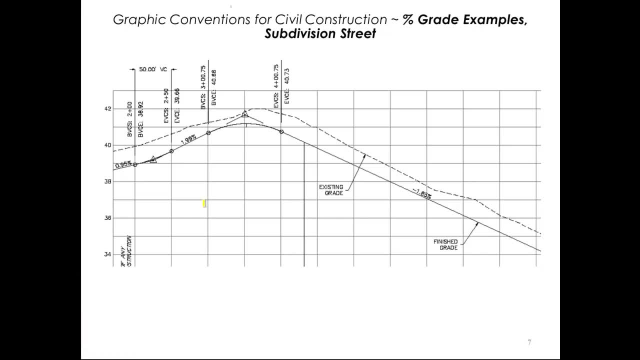 a pretty gradual slope and let's see if we can figure that out. this is a one point nine nine percent slope, so that's essentially two feet and a hundred feet. that's not really very steep when you think about it. there's a change point here. this is a point nine five percent slope, or just under one foot per. 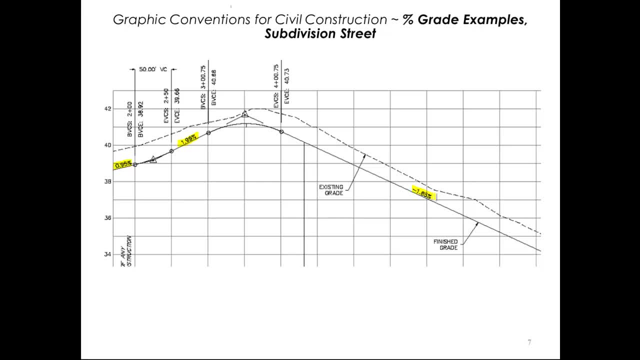 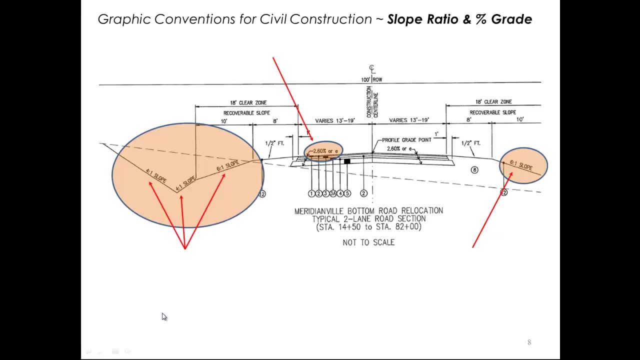 hundred, and then what looks like a really steep hill. here is simply one point eight five feet per hundred feet. this is a typical road section and in this case we're going to see how both the slope ratio for shorter, steeper gradients and the percent grade for flatter gradients can be used to fully illustrate the 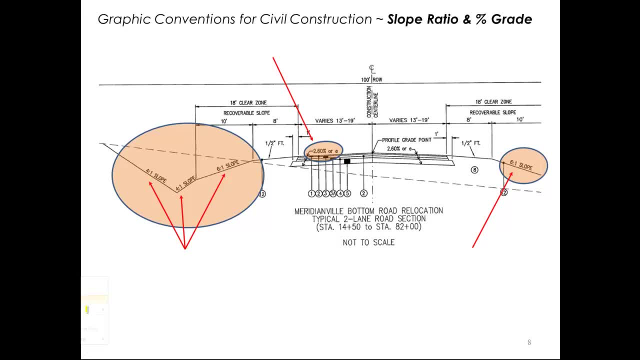 work. so over here on this side, we're actually into a cut situation and we can see that a ditch is to be excavated to drain the water. on the side of the road- and let me get a different color here- we see a four to one slope. we see a. 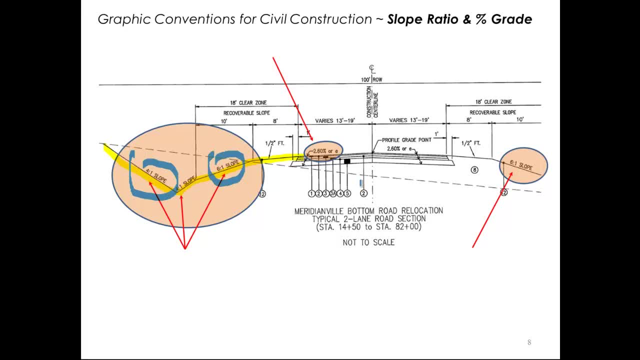 six to one slope. over here it's already circled in blue and if we look at the top surface of the road itself right here and right here running out to the shoulder, we can see that that is at a two point six percent slope, or two point six. 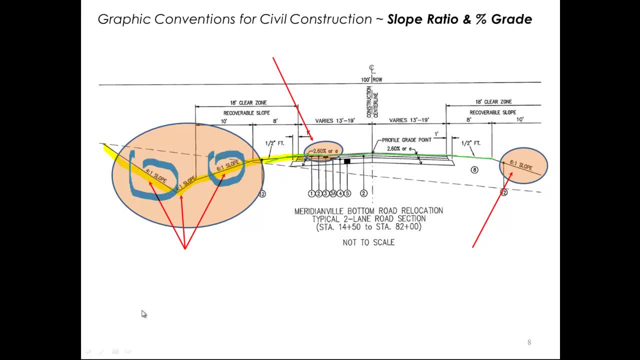 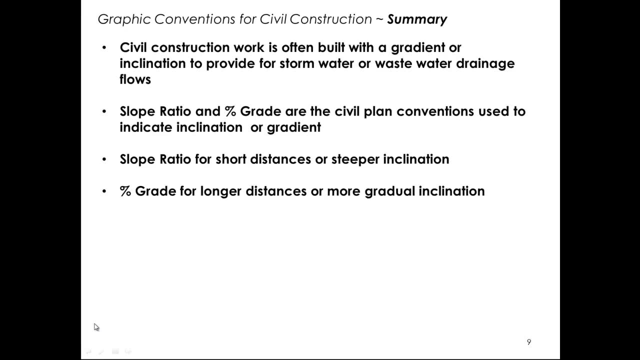 feet per hundred. Let's summarize what we've learned, then, about slope and grade. Most civil work is inclined or at a gradient to provide for the flow of water. Our two conventions, slope ratio and percent grade, are used to define the required inclination of the work. Slope ratio: